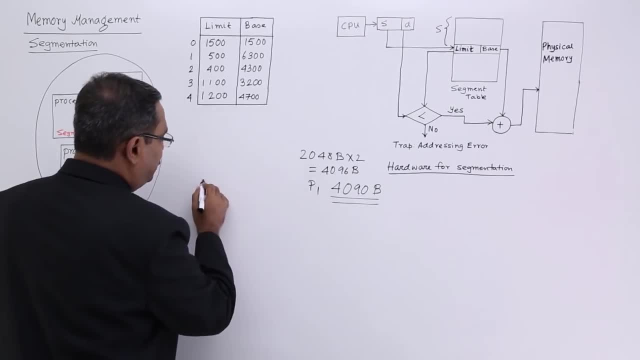 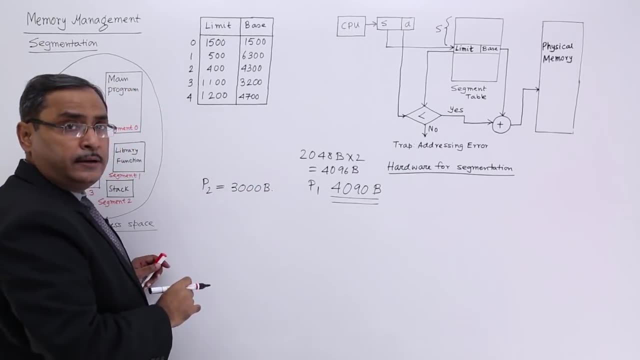 size is this one and one process, let it be P1.. Say another process, P2 is having got a size, of say, 3000 bytes. then what will happen? 2048 bytes will be there in the page 1.. In. 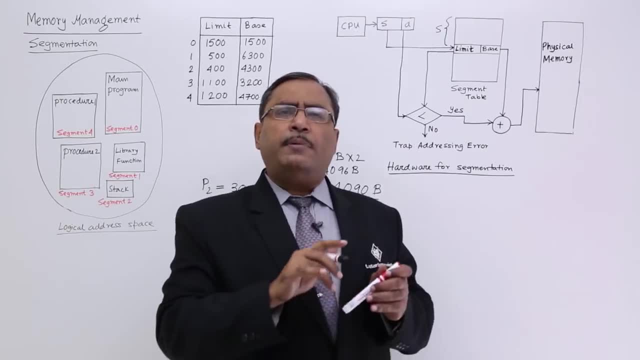 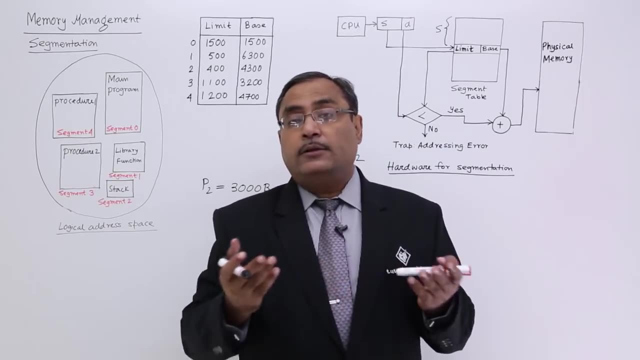 the page 2.. So so many bytes of free spaces will be there, but I am having no option because I said to allocate page size wise or frame size wise. I am not having any other option. So so many bytes of free spaces will be there in the respective frame where this one particular 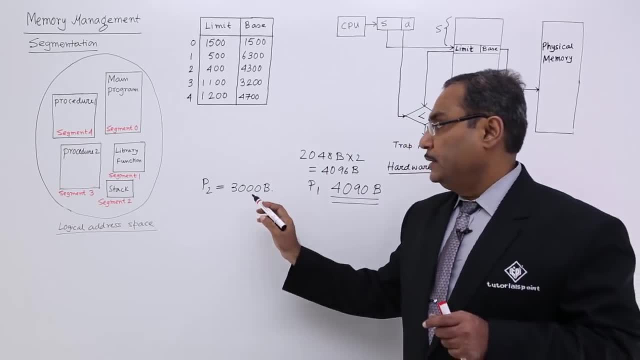 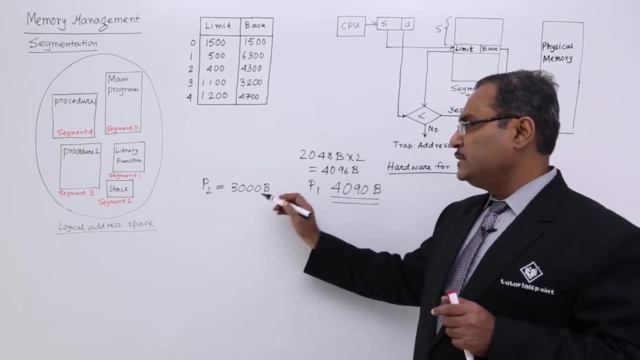 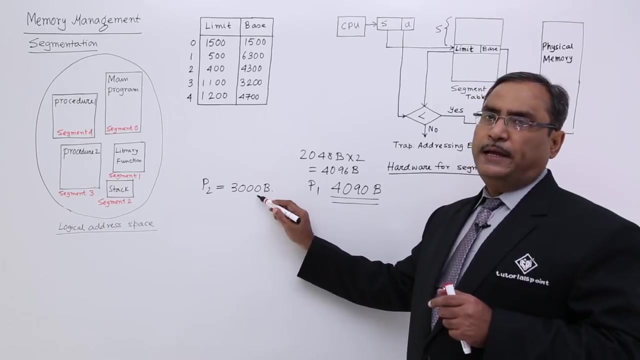 page has got loaded. the second page has got loaded. I think you are getting my issue. So 2048 bytes for the frame number for the page, the page size of the frame size, but my process size is this: one page will be completely filled up with 2048 bytes but in the second page it will be having 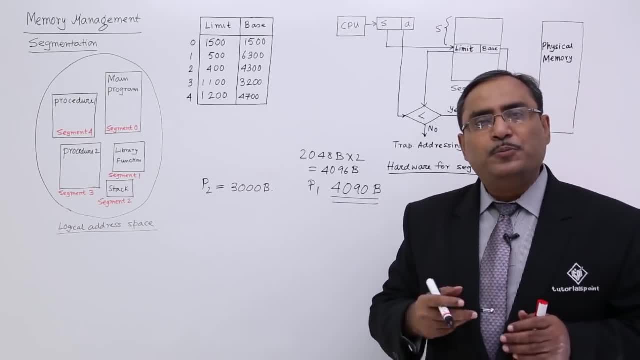 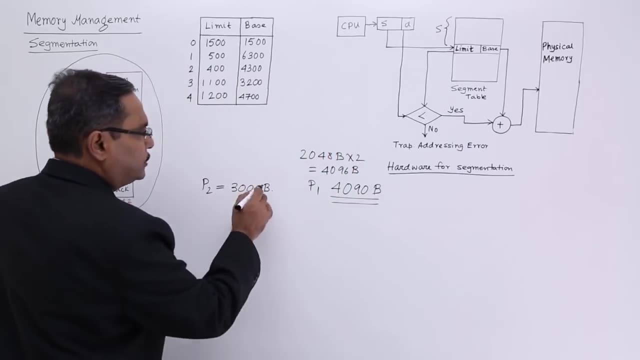 952 bytes of free space will be there, but in the page map table it will be written that it is completely ok. ok, So that will be. that will be occurring here. ok, Now see, So I am just telling in this way: 2048. So 2048 will be occupied, and then 2048. 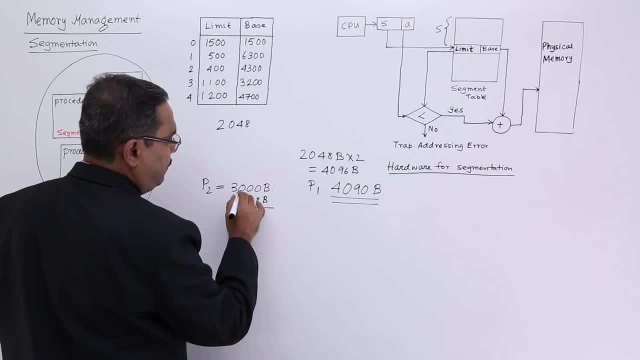 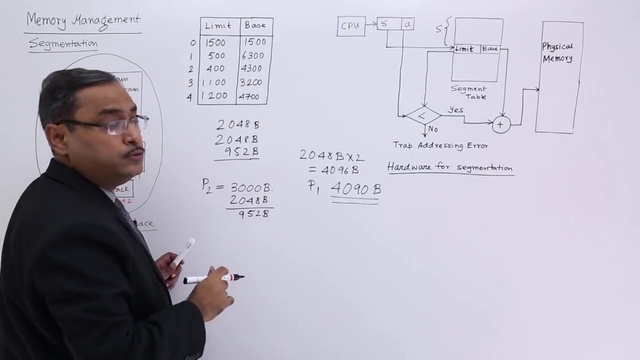 will be subtracted from here. I am getting here 52,. I am getting here 9.. So 952 bytes will be loaded in the second page. So how much free spaces will be there in the respective page that will be used? So it will be 6, this is my 9 and this is my 10.. So 1096 bytes. 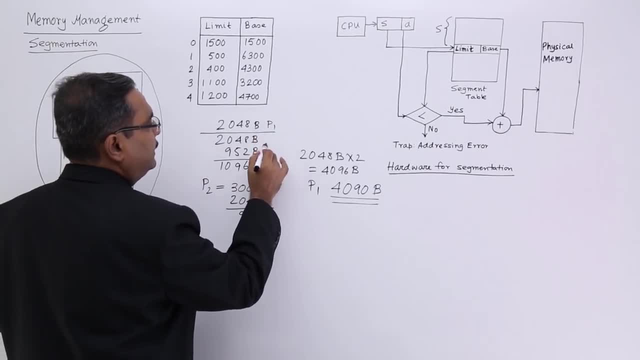 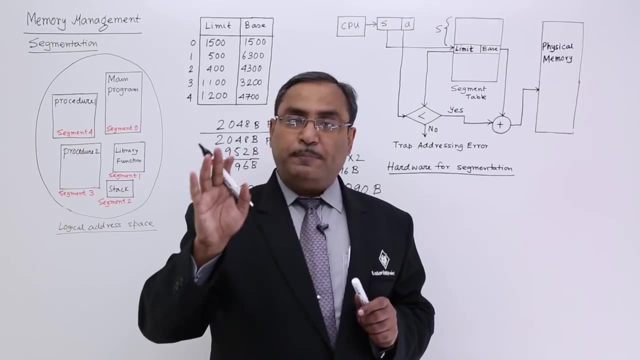 of free space there in the second page. this is the page 1, let it be. let it be the page 2.. So that amount of space will remain vacant in the page 2, but in the page map table I shall write that 2 frames have got allocated. So that is the main disadvantage in case. 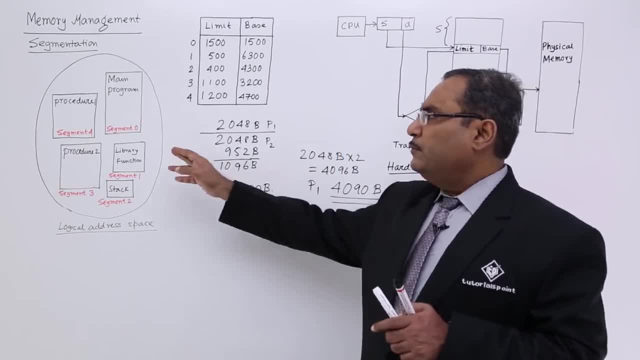 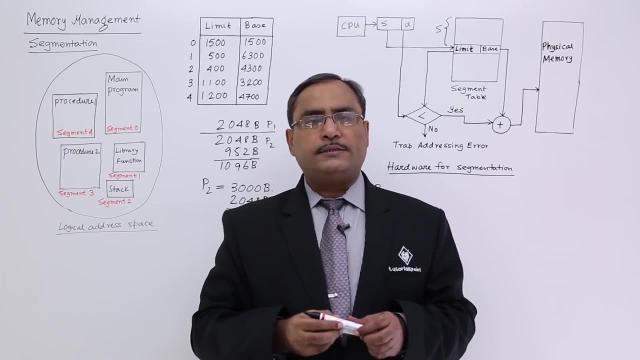 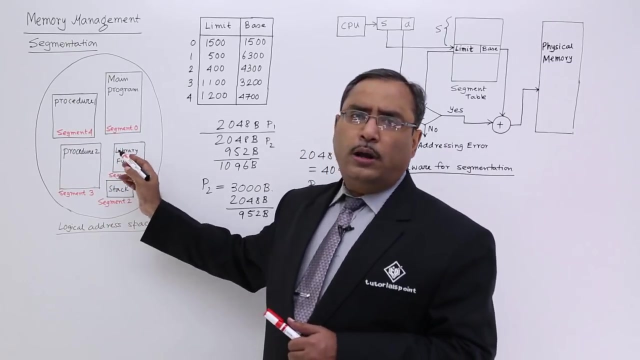 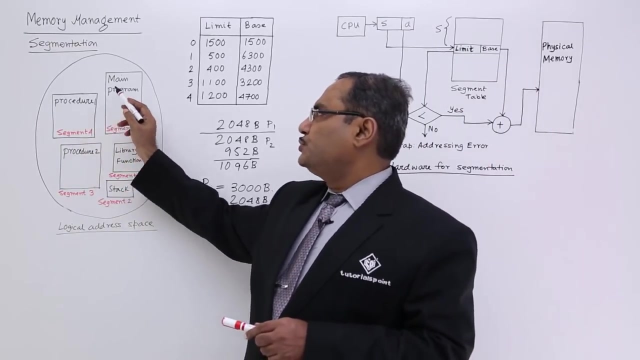 of paging. So to solve this problem, we are going to introduce this one, that is, our segmentation. How does segmentation work? Let me discuss that one right now. Now, in case of segmentation, let us suppose that is the program. So we have 5 segments, segment 0 to segment 4 containing procedures, containing the main. 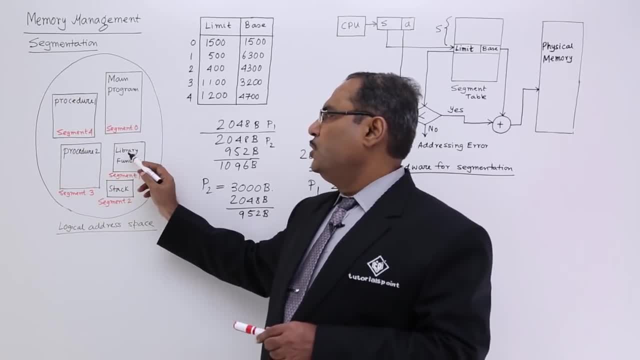 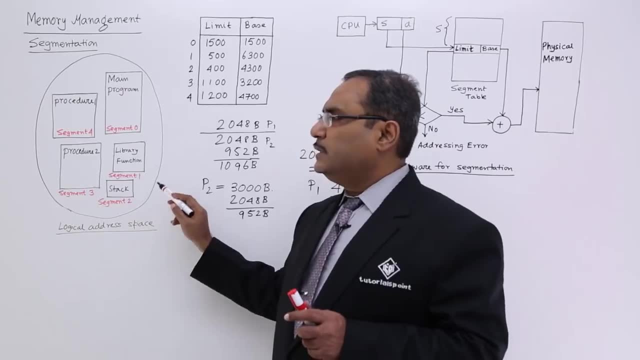 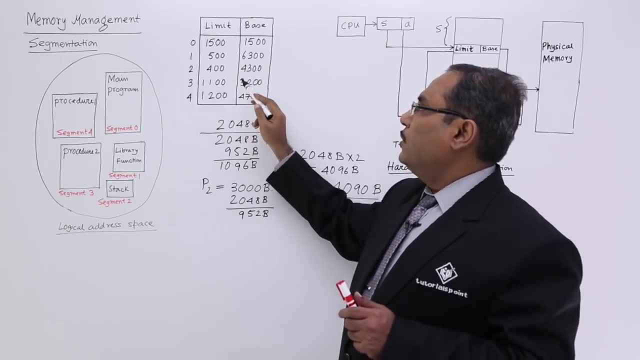 program body containing another procedure, procedure 2, containing the library function. body containing the occupying the stack. So these are the different segments are there in a program and the respective segments, that limit and the base address have got mentioned. What is the limit, That is the segment size and what is the base address from where it? 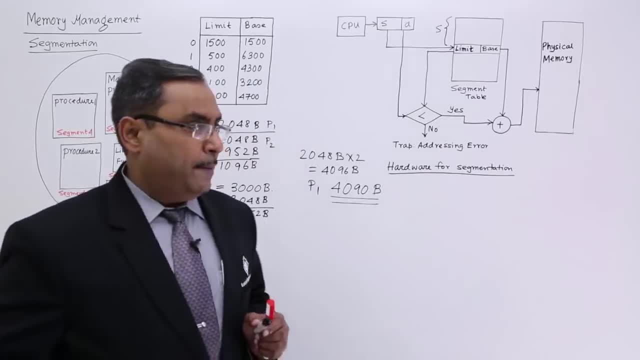 has to be loaded in the computer system. So that is the base address. So that is the maximum space in the program that we have collected, and the minimum number of member elements has to be taking into account. Fraternal is whether or not there is a maximum space. 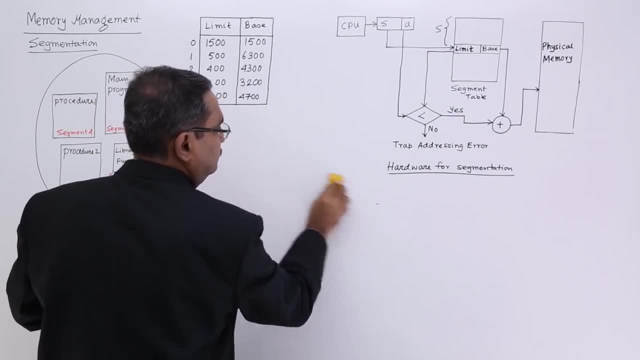 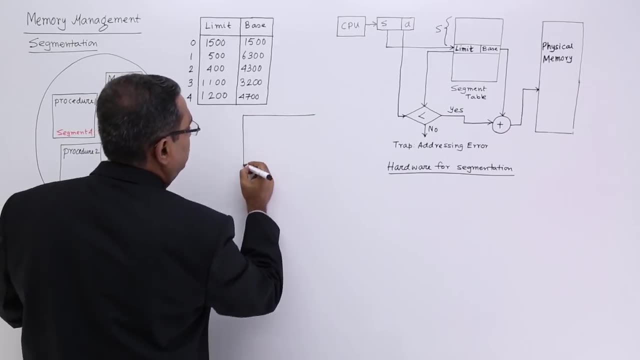 space. What is the minimum stack size volume? So the maximum of them is herself. What is the minimum size then of her? She is standing here now. she sits here. she has struggled to write a rupees 1 upon rupees 2.. 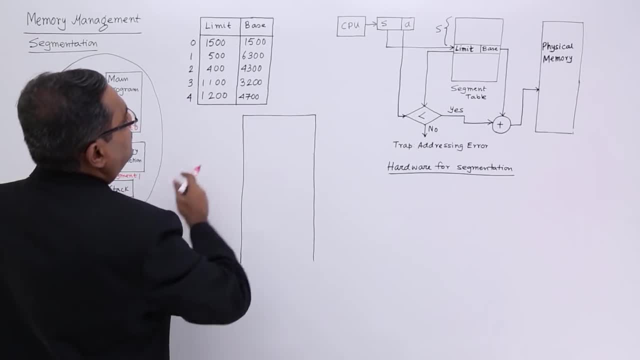 So there is rest of theYUO because she is arriving the computer system. You do not have a maximum space space, Take it anywhere else, Take it anywhere else. and If I refer to the other person, I have written인데요 dollars, a object, 2ش Van wall, from where she is, 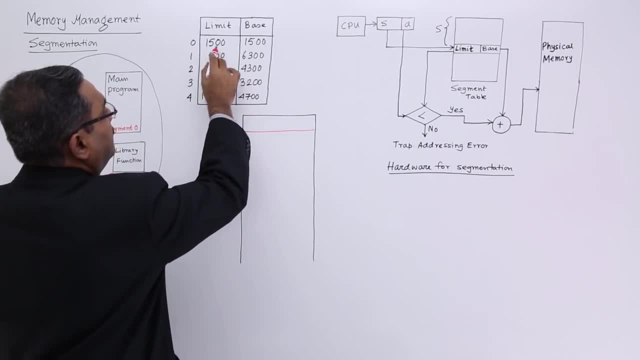 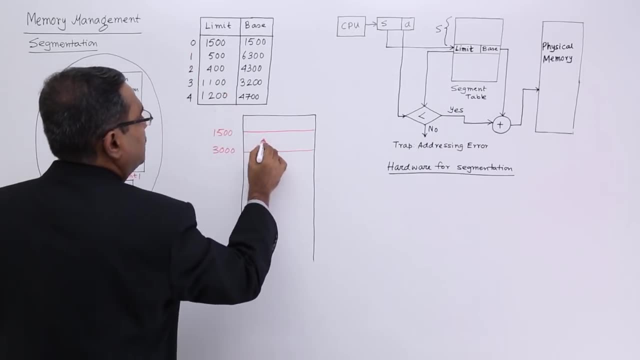 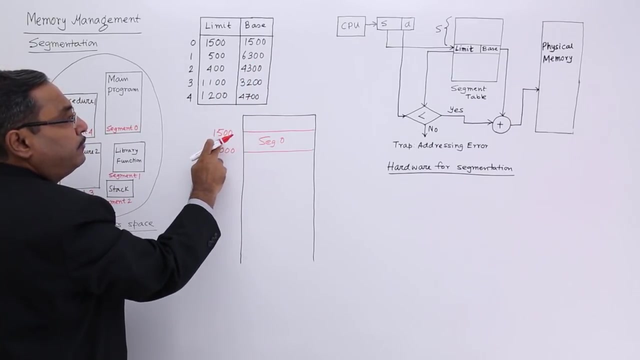 coming into the computer. the base and limit will be 1500. so that means up to 3000 segment number 0 will get loaded. i think you are getting my issue. base at this is 1500 and limit- that is, the size- is 1500. 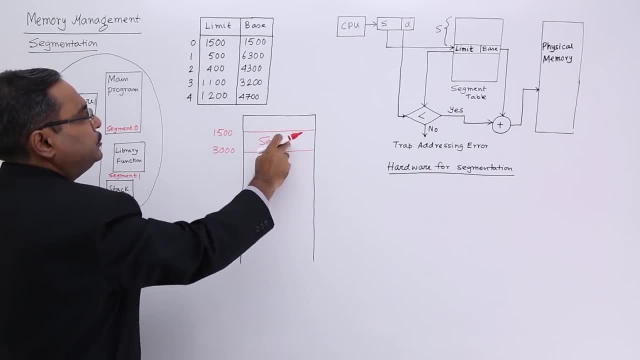 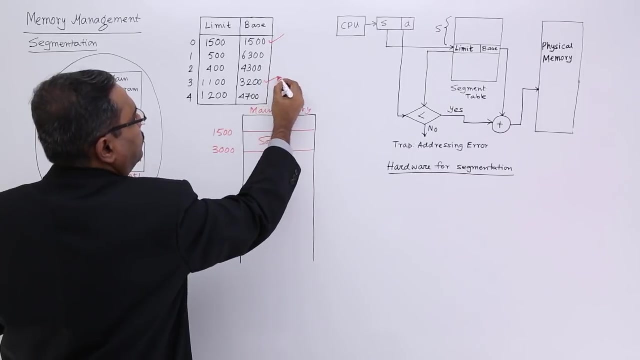 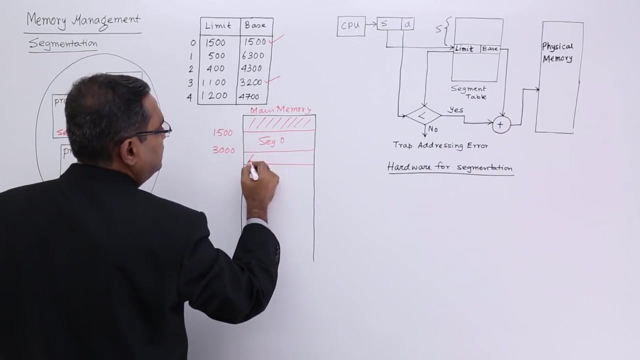 so that is why, from 1500 to 3000, segment number 0 will be there in the main memory. ok, now what is the next address? i think this one. so it has got loaded, so i shall go for this. that is 3 2 0, 0, so the it is a free space or other programs might be existing. ok, now. 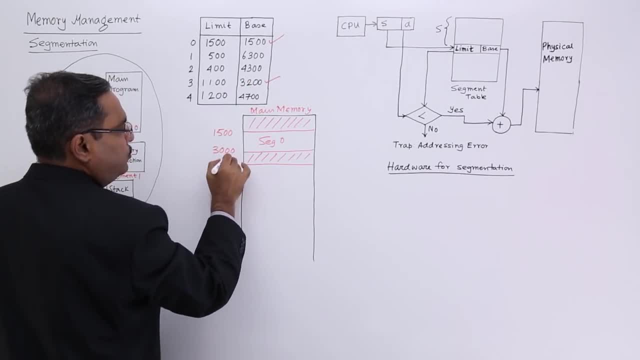 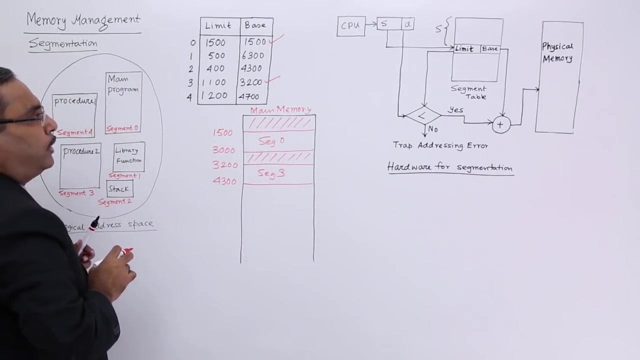 so it will be starting from 3 2 0 0, so 200 bytes of free space here, and it is having a limit of 1 1 0 0, so it will be terminated at 4 3 0 0. which one? that is a segment 3. that is a segment 3. ok, what is the next address? 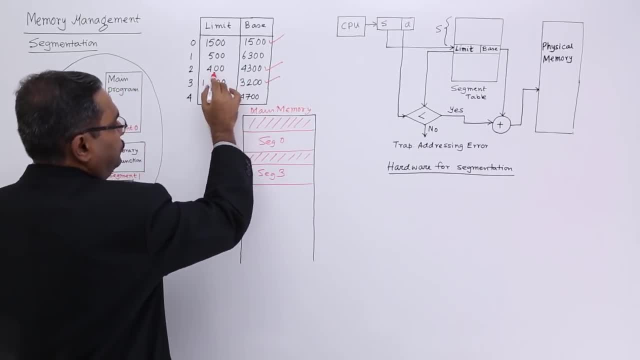 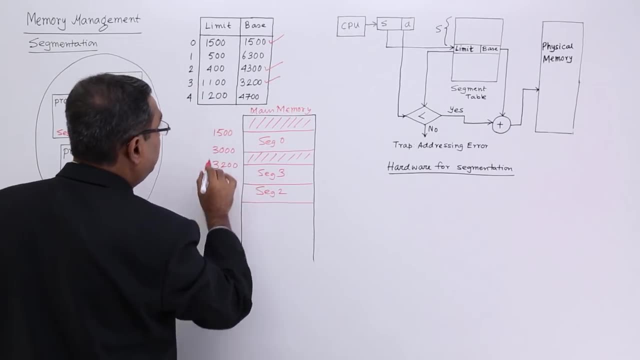 that is 4 3 0 0, so i am taking this one. so 4 3 0 0 400 and that is for. that is for segment number 2. so segment number 2 will be there. 400 is the limit. 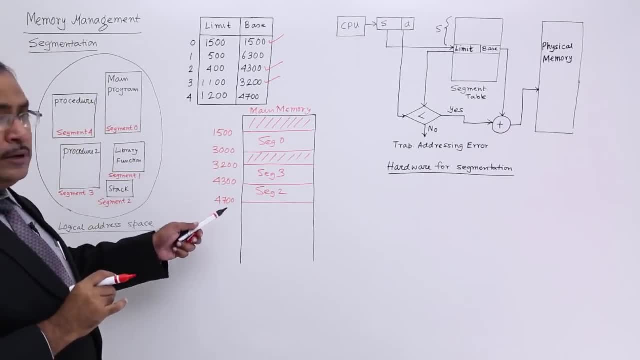 so that is for segment number 2. so segment number 2 will be there. 400 is the limit, so it will get end at 4 7 0, 0. i think you are getting this one. so 1500 to 3000, that is 1500. 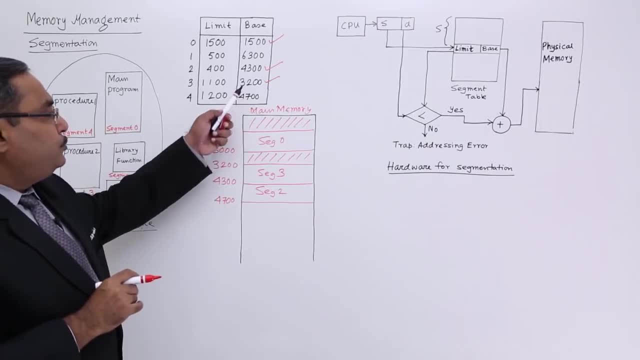 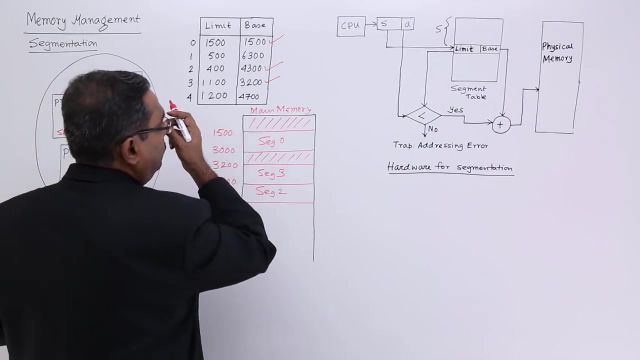 is the limit for segment number 0. it will be starting from 3 2 0 0 and then it is having a size of this, so it will get terminated here. but that is the starting address of segment number 2, with the size of 400. so it will get terminated as at 4 7 0 0 and then i shall 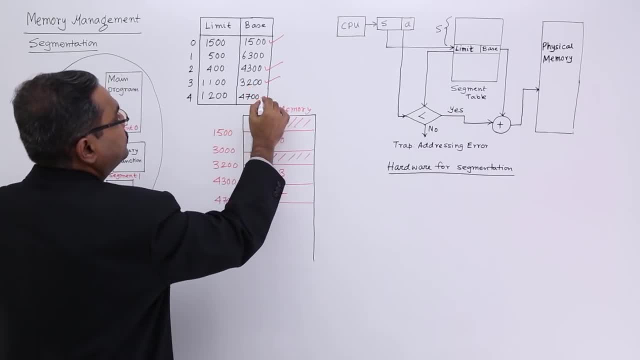 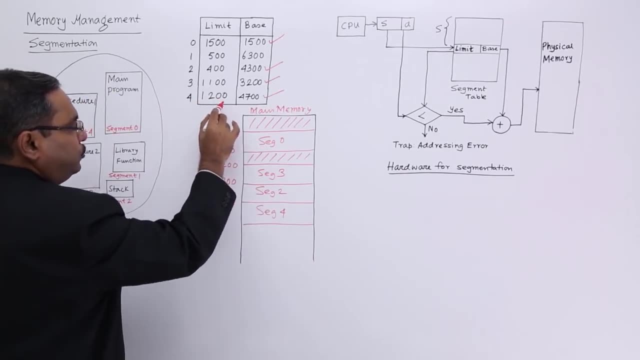 go for which one? 4 7 0 0, 4 7 0 0, which is this one? so i shall go for segment number 4. i shall go for segment 4 and it is having a size of 1200, so 59, 00 will be the size for. 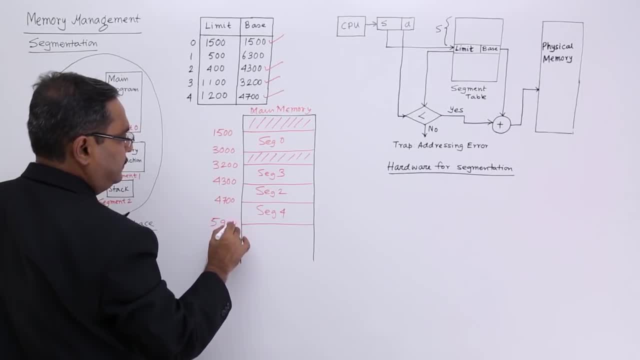 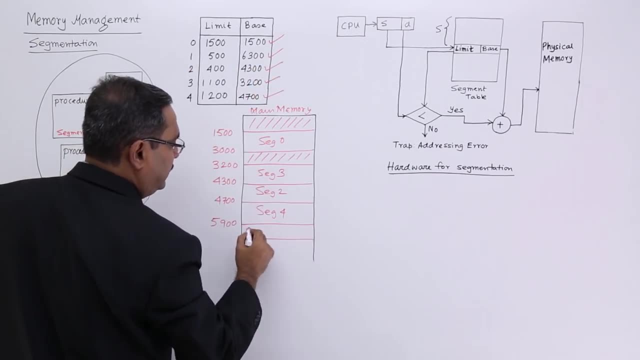 segment number 4. so what is remaining remaining is segment number 1, so segment number 1. so there will be some free space here in between. so segment number 1 will be starting at 6, 3, 0, 0. so segment number 0, 1, 2, 3, 4. all of them have got 1 0, 1, 0, so i will go for segment. 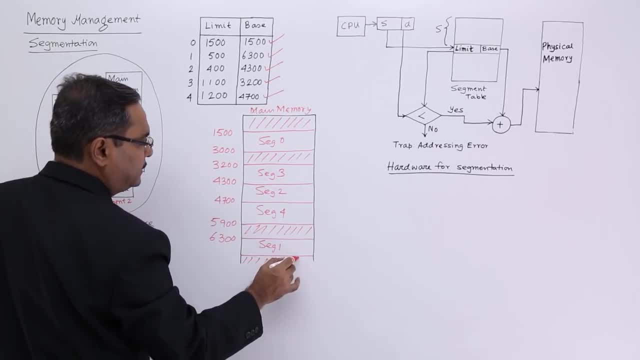 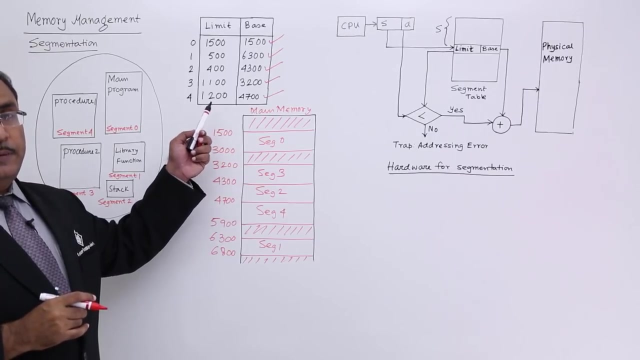 4. part loaded. rest part will be the free space. segment number 1 is having a size of 500, so 6800. at this location it will get terminated So in this way. this is the segmentation table, or segment table. this is the segment table and this is the memory map I have shown you. 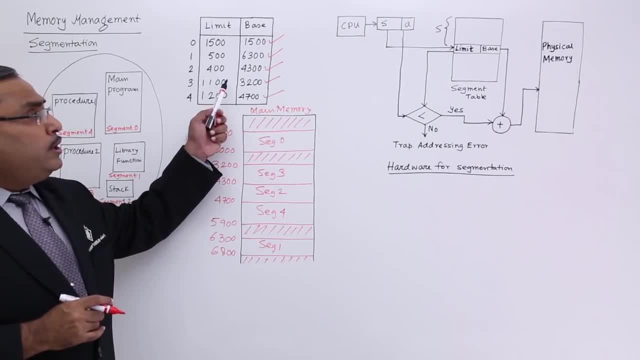 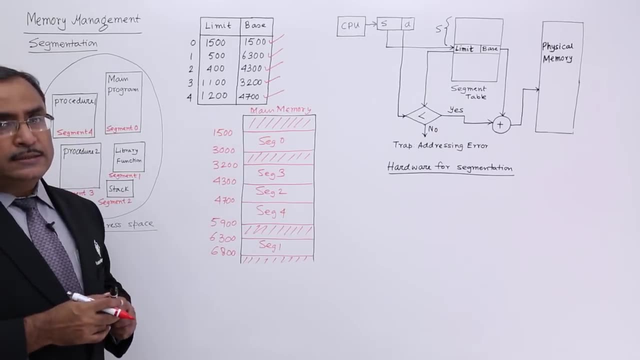 that how this segment table is holding data and how the memory map is taking place. So every problem comes in this particular, from this particular concept. you should have to answer accordingly. So segment table is having two columns. segment table is having two columns. what is the column That is one? is the limit limit means what? 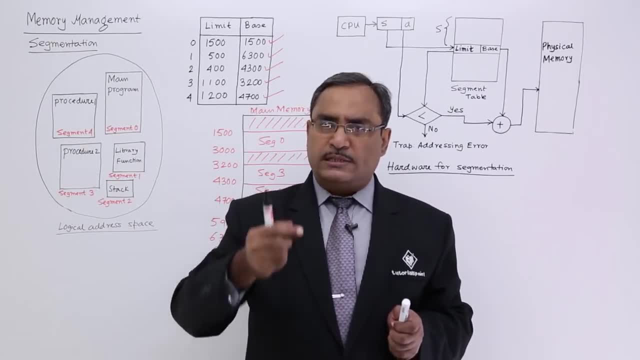 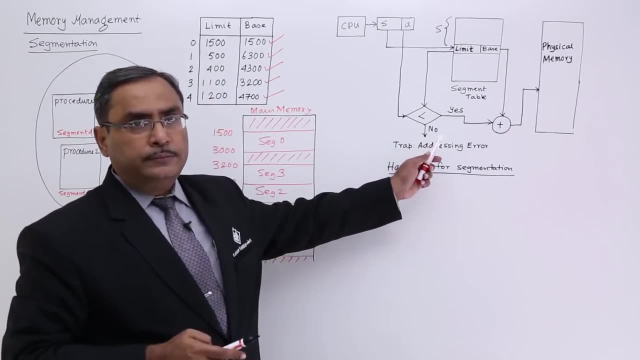 Size of the segment. what is the other one? Base means what Means the starting address of the segment in the computers memory. so it will be coming like this. So let me show you the required hardware. So CPU will produce a logical address. so this is my logical address.